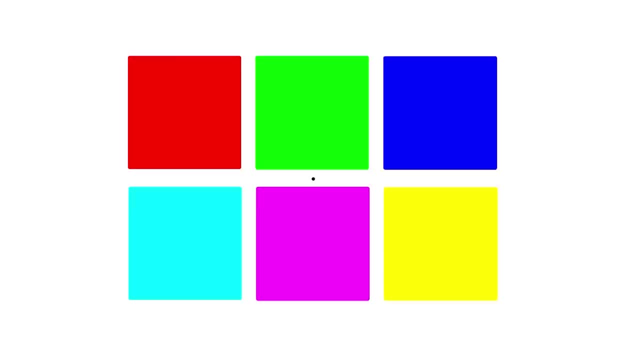 are really similar. This is what I showed you, So let's try to compare them and see where you find a good complement. You will find different colors of each color wheel. The colors are complementary and for about 20 to 30 seconds, When I remove the square, I ask you to keep your eyes on the white. 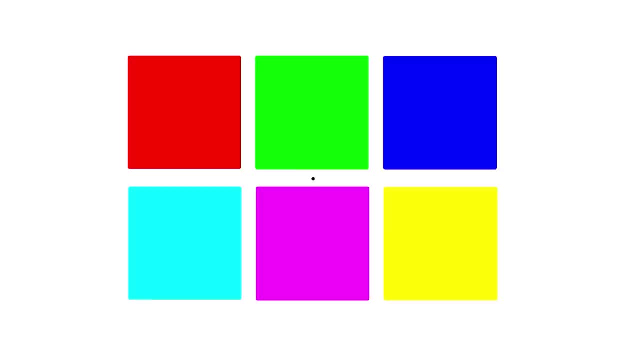 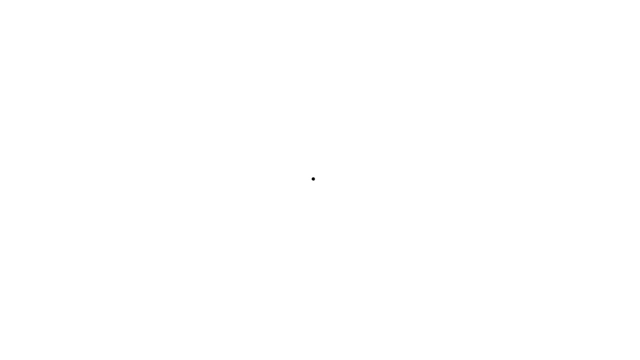 background. If you want, you can let your eyes blur out. Now keep your eyes centered. don't move for another 10 seconds. Now you should see a persistent square appear. This is how we define the visual complementary color And, in case you were wondering, this is not an effect of your screen. 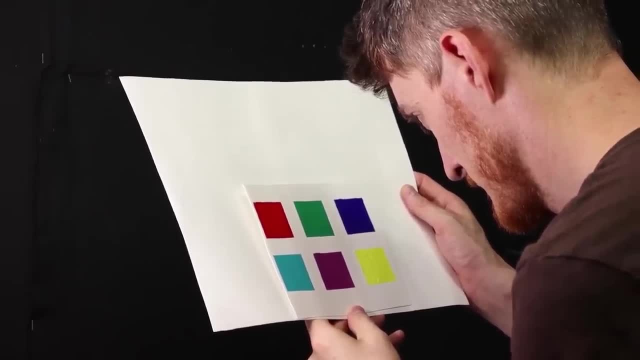 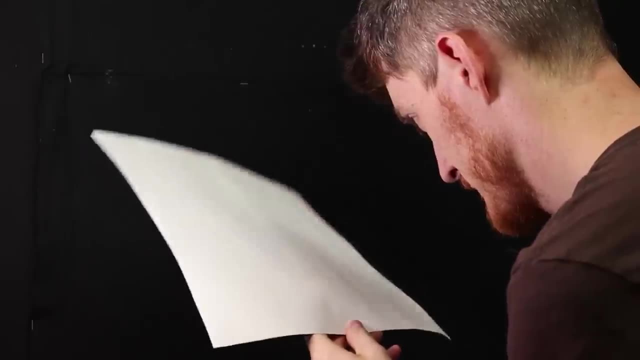 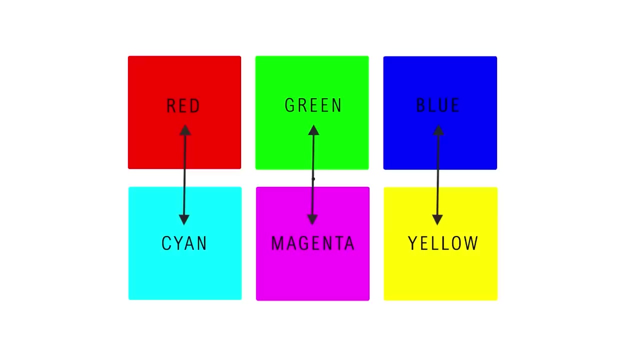 you can do the same experiment with paint on a white surface. The phenomenon of visual persistence is an effect of our visual system. by having the same color on screen And with paint. here are the approximate complementary couples that we get: Red complementary to cyan, yellow complementary to blue. 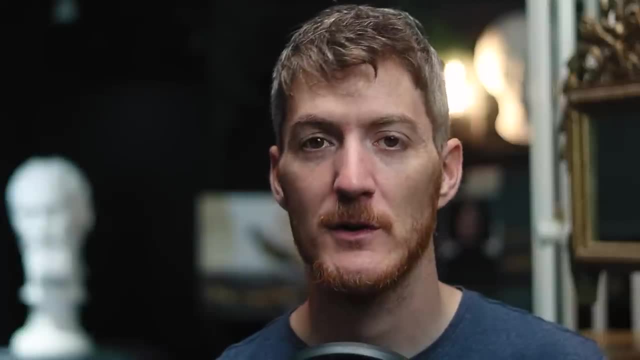 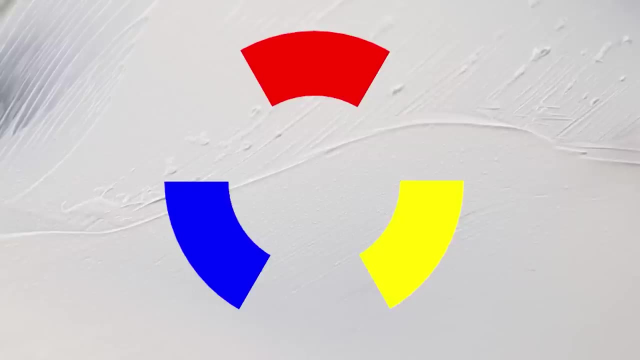 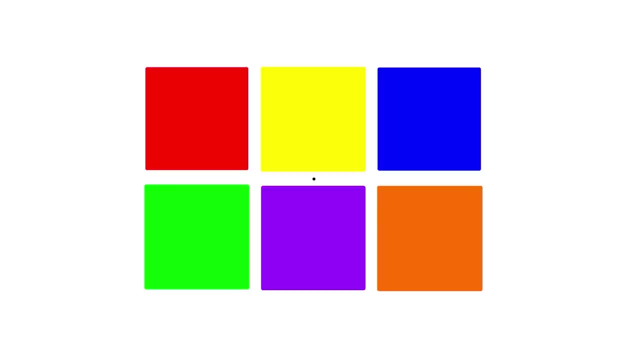 and magenta, complementary to green. It should be noted that these pairs do not work in a model where red, blue and yellow are primary colors. In this one, the supposedly complementary pairs are red and green, yellow and purple and orange and blue And, as you can see, they do not match and they do not match the same color. As you can see, they do not match the same color, But they do match the same color And, as you can see, they do not match the same color And do not really match the observations. 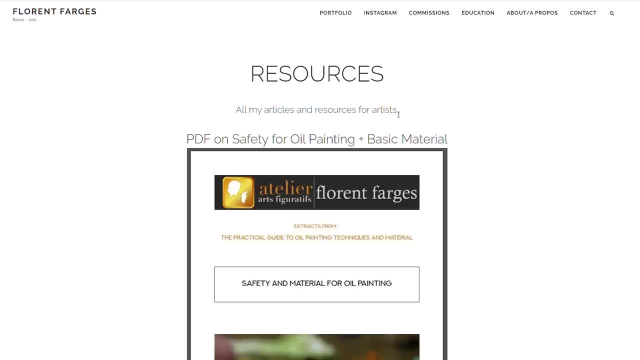 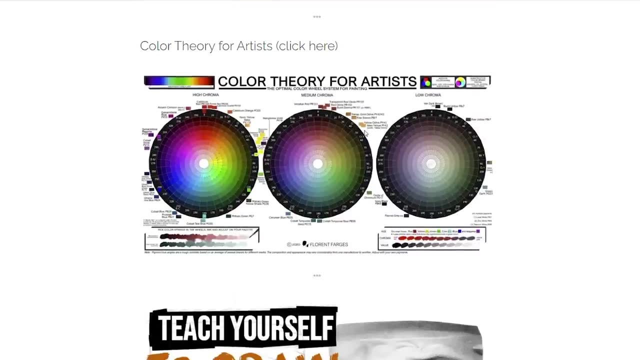 To follow this video, you're going to need to have a look at my color wheel that you can find on my website. The free version is a direct PDF download, straightforward. No email, no mandatory subscription or anything like that. It's a simple download. 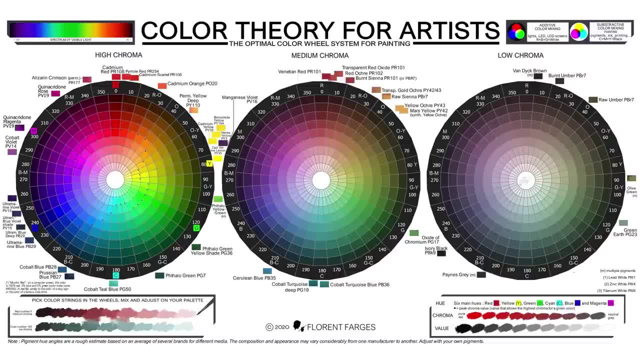 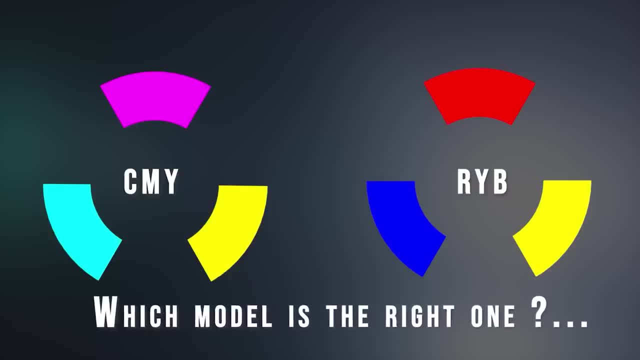 I'm going to use this color system as my reference for the rest of the video, so make sure to just have a look. However, our previous question was: how can we be sure that we have the right complementaries? We've seen how, but regarding color harmony though, 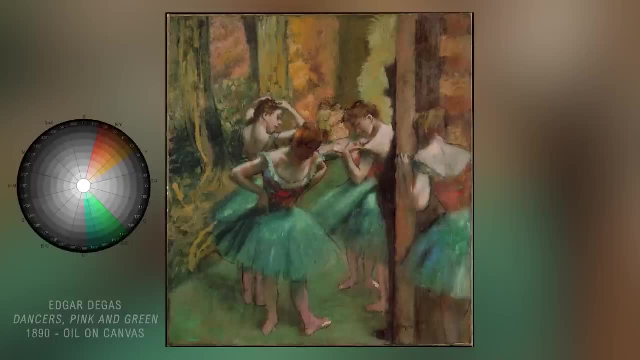 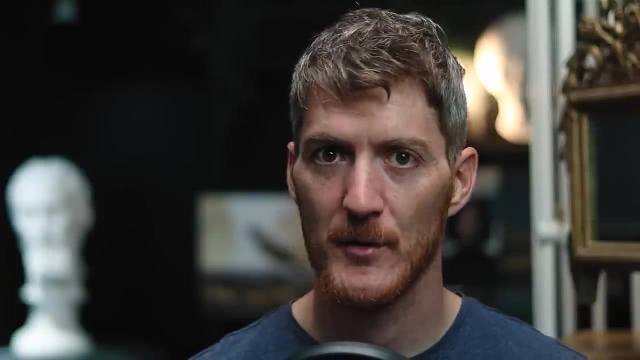 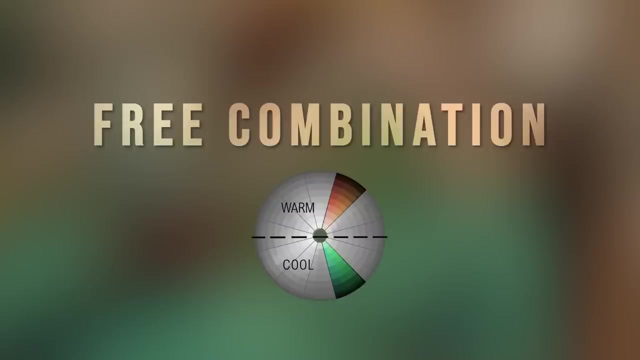 we need to be a little bit more nuanced. Two colors don't specifically need to be exactly complementary to be harmonious. In fact, with two colors, the margin is pretty wide. Any two colors can act as complementaries if they are more or less on the opposite side of the wheel. 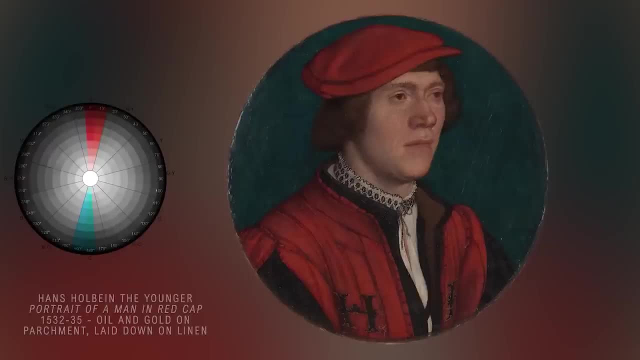 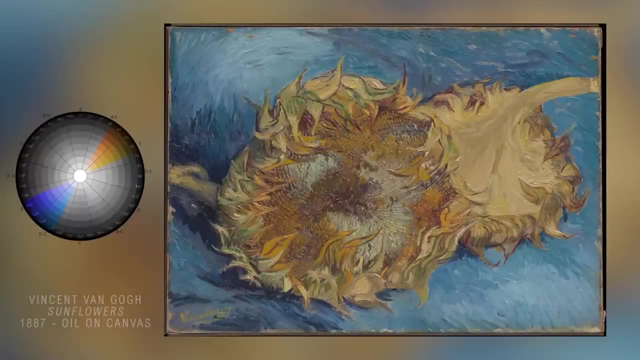 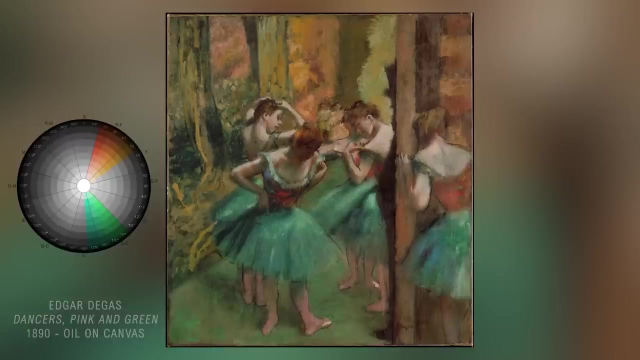 They don't have to be perfectly aligned with the center of the wheel to work fine, They will just make a dynamic opposition whatever they are. Using only two colors offers a complete creative freedom in the choice of hues. Basically, a two color composition functions. 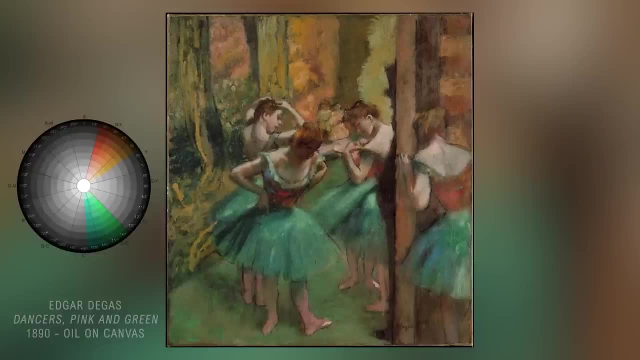 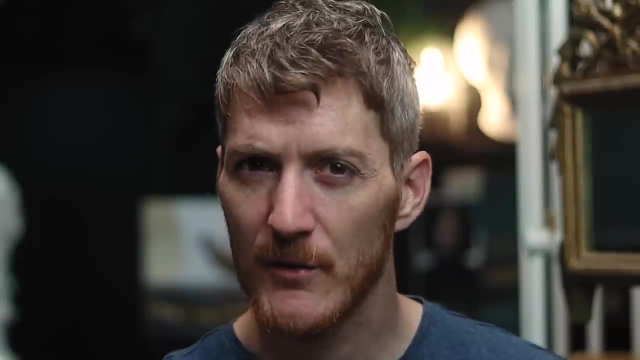 like a black and white image, but with colors. The tighter the range, the more it will work like a black and white picture with a clear focus on values and shapes. Of course, there would be so much more to say about complementary colors. 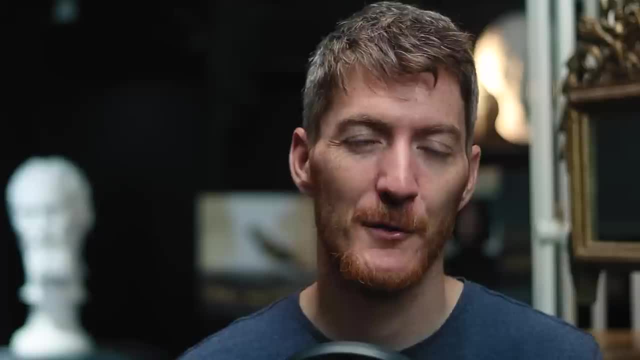 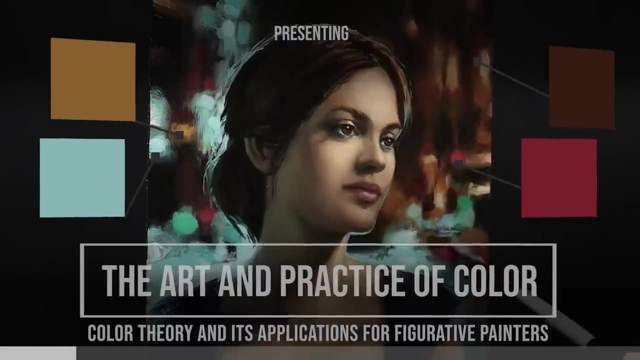 The thing is that with color theory, the more you learn, the more there is to learn. If you want to go further and explore these topics more in depth, and specifically the connection between theory and practice, you can check out my course and if you want to. 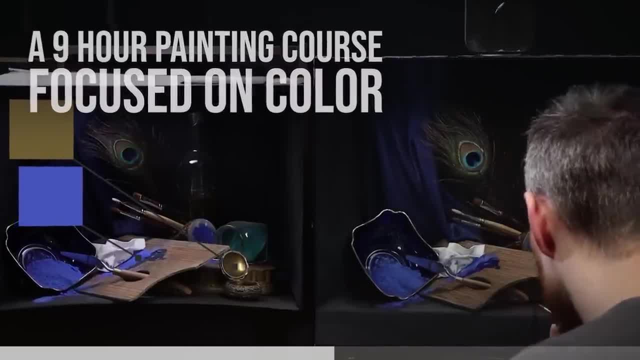 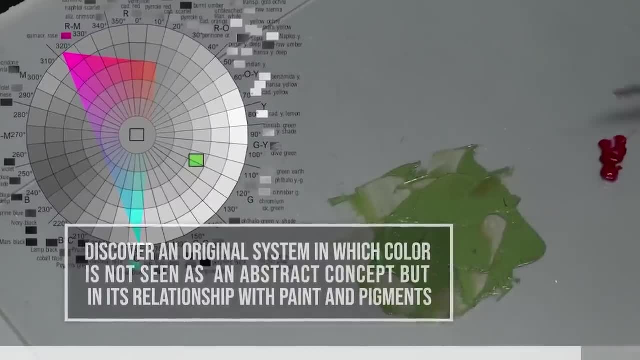 learn more, you can just follow the link below. I also have an oil painting course that covers all the technical aspects from start to finish and might help you as well, But for the moment let's just go back to the video now. Dominant Tonic Accent: When you have three colors and then all of 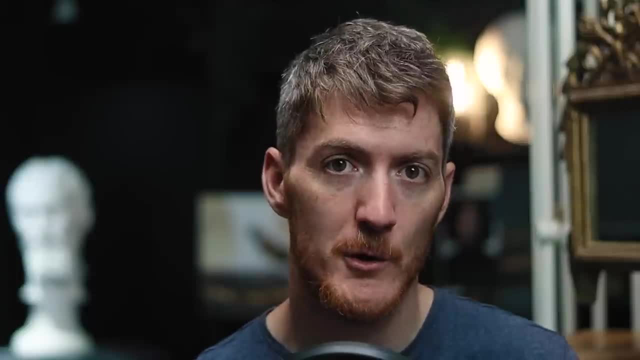 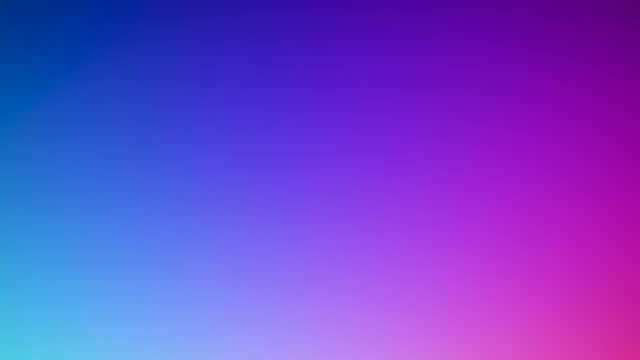 a sudden, it's a lot harder to paint them together harmoniously. Just to be clear: when I say three colors, obviously there are millions of nuances of colors, as many as one can count actually, but by three I mean three groups of shades. 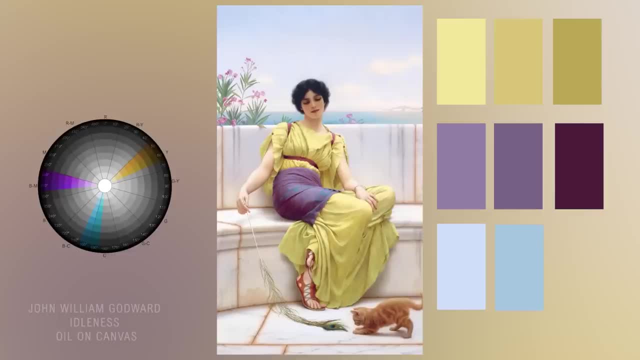 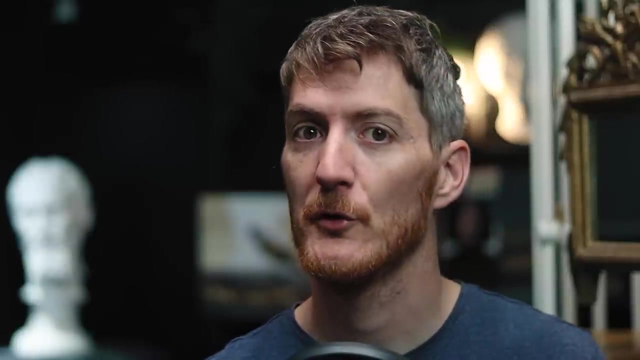 of the same hue. The word color is not a single shade, but a small range of shades. So, as I said to compose with three colors, the key is to understand that what matters is not only the hues that you choose, but also the chroma and the value of those hues. 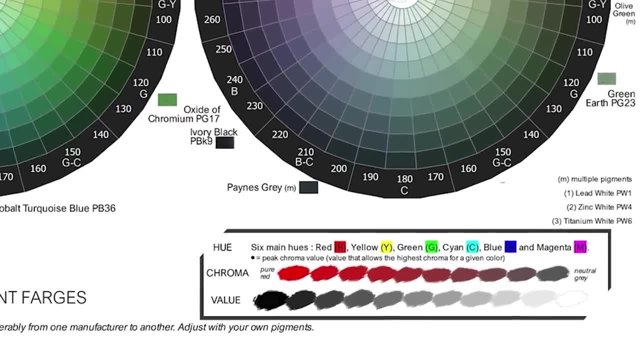 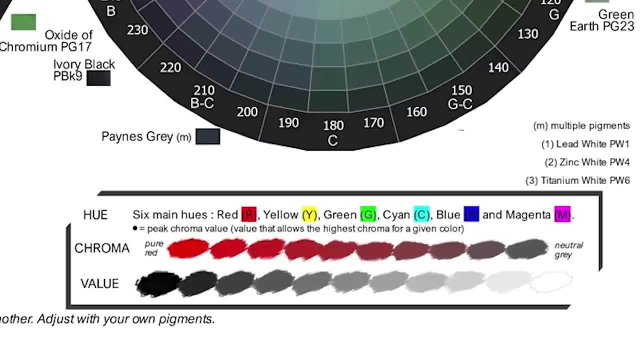 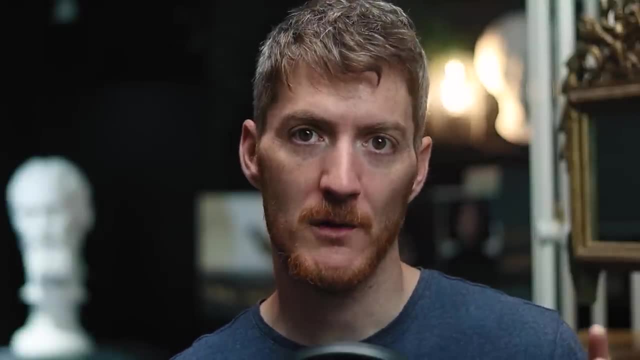 If you need a reminder of what those are, refer to my color wheel picture or see any of my previous color theory videos on my channel. Chroma is certainly the most important notion to take into account when thinking about composition, especially with three colors. 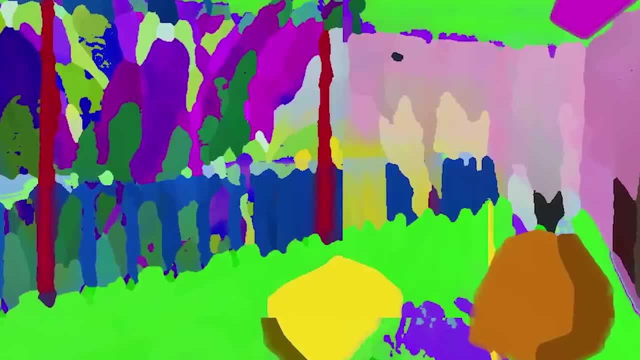 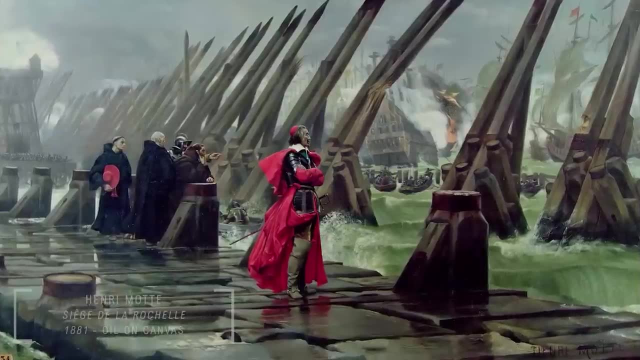 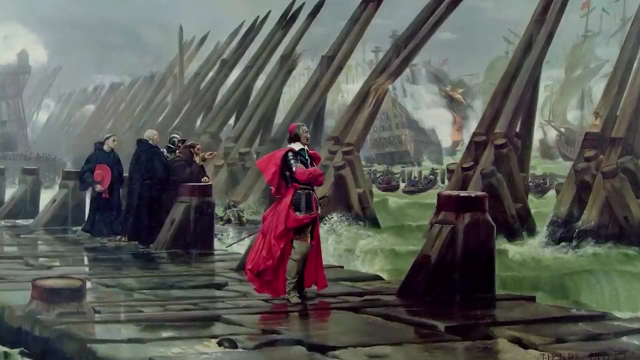 Indeed, if all colors have a high chroma, the overall impression will quickly become very unpleasant. On the other hand, if most colors are rather mute, but only one touch of a strong vivid color appears, the eye will naturally be attracted to it. 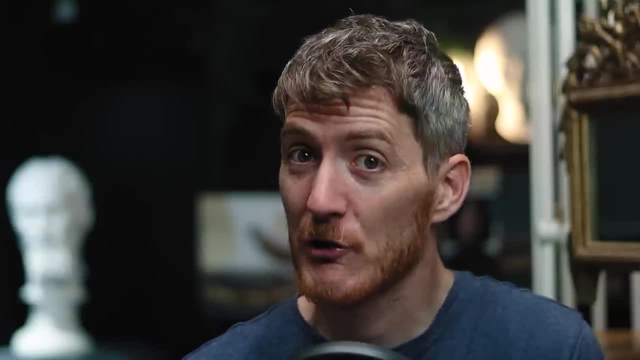 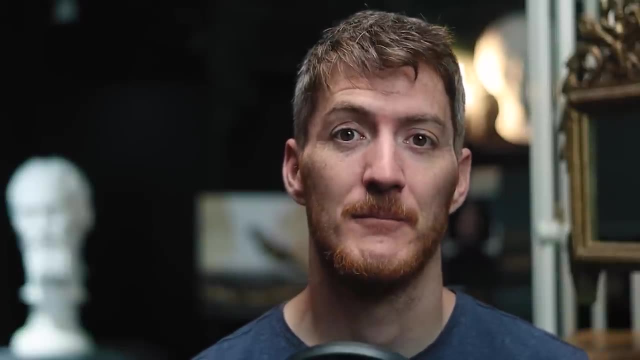 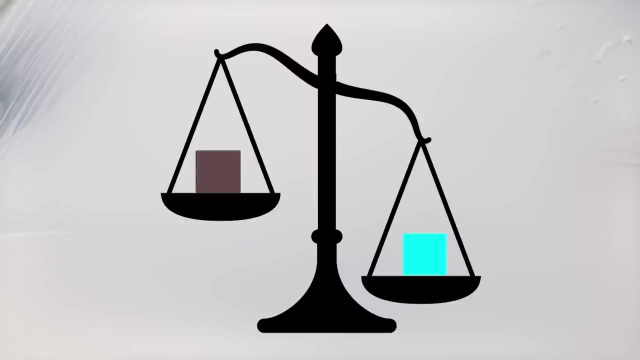 Chroma is a little bit like sugar for the eye and, as with the sugar, the taste is better if it's not excessive. As you might expect, it's all about balance. Imagine a weigh scale: On one side a very dull color, on the other side a very vivid chromatic one. 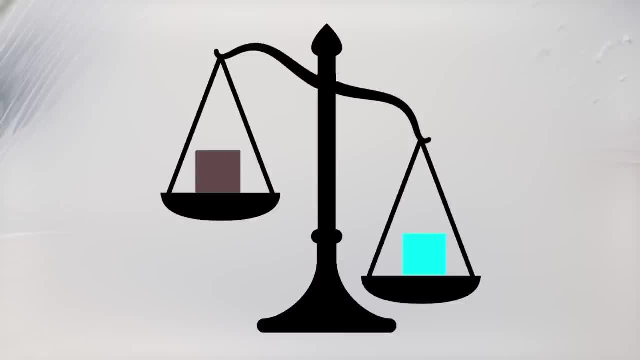 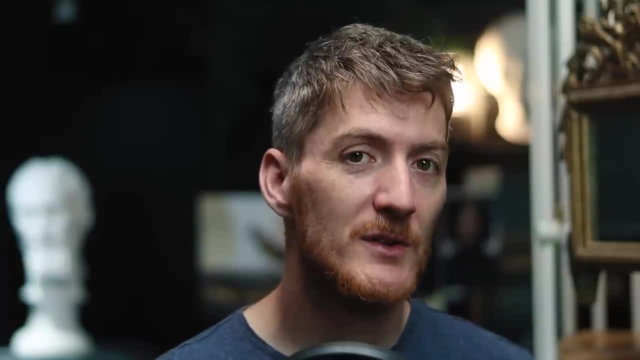 The latter will make the scale weigh on its side. To regain the balance, the duller color has to be larger and take up more space. You see that the issue is not just the choice of the color and the chroma, but also the 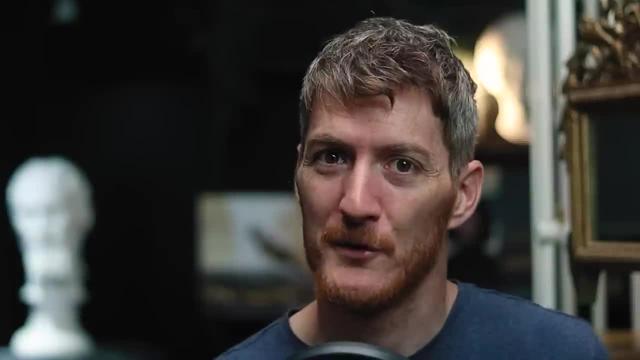 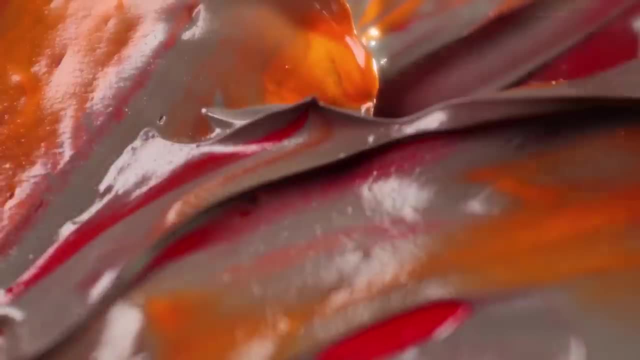 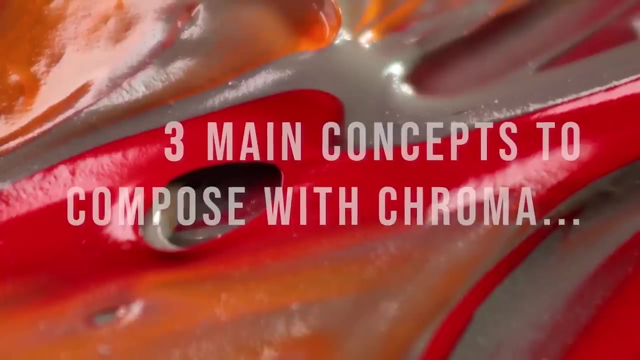 space it occupies And it's importance in the composition. So how to harmonize these notions easily? I'm going to share with you a system that I've created, inspired by music, to remember these main concepts. I have not invented anything, just the words to keep them in mind and remember these concepts. 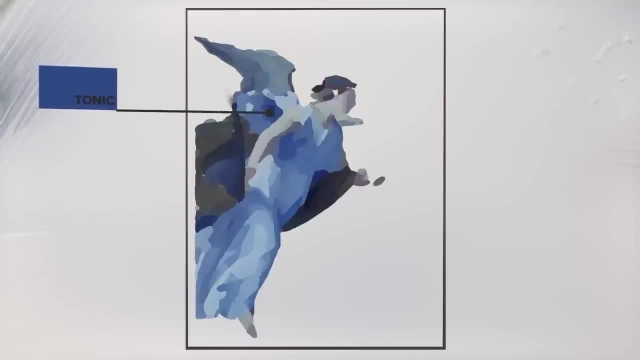 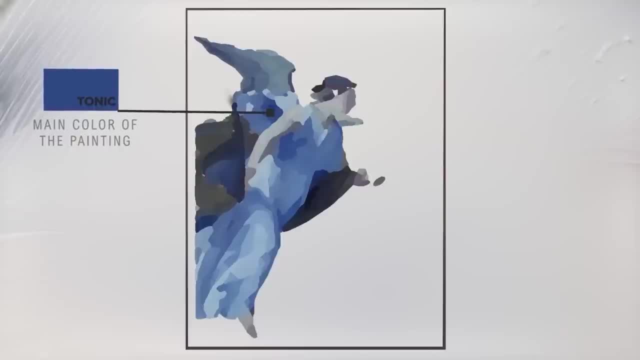 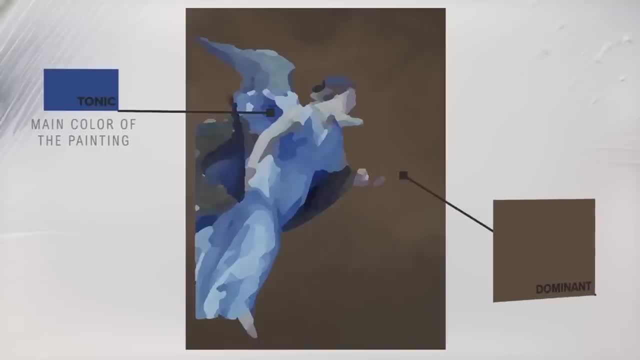 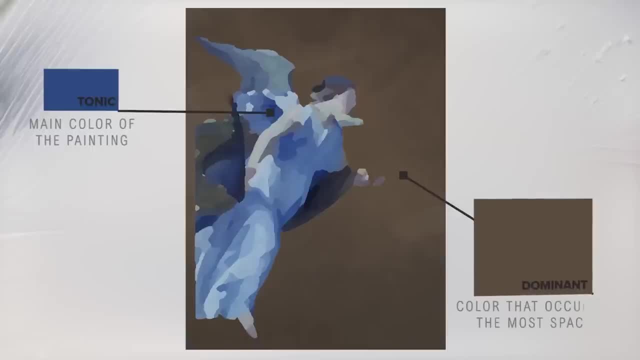 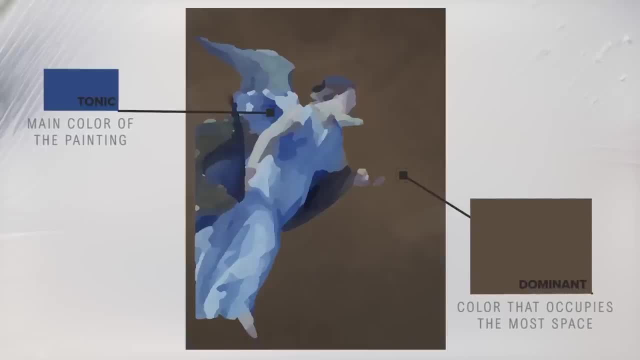 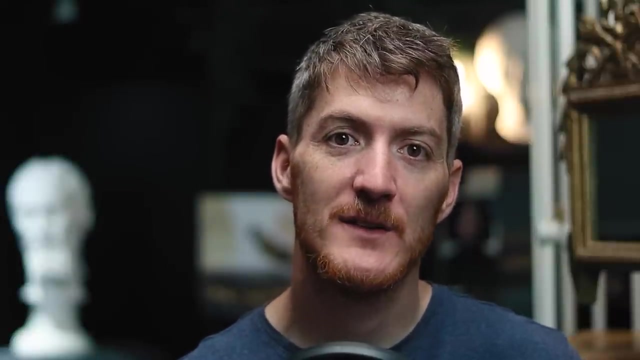 The one that first comes to mind: dour and more mute. 3. The accent: It's a small touch of color with a small surface area, supposed to just attract the eye and bring a little punch to the picture. What defines an accent is that it's not a structural part of the 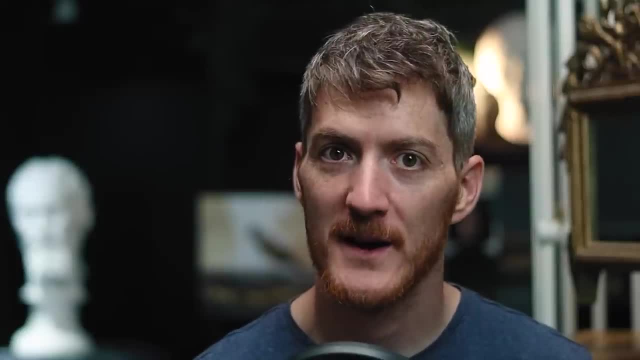 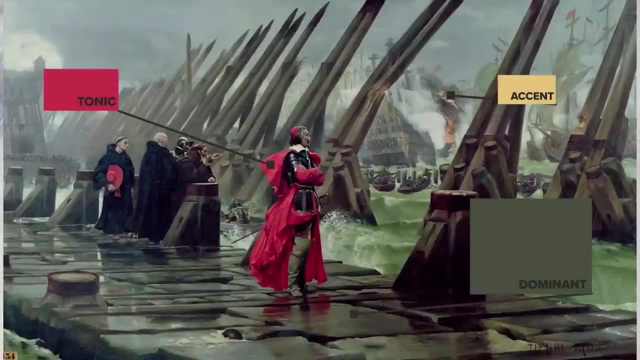 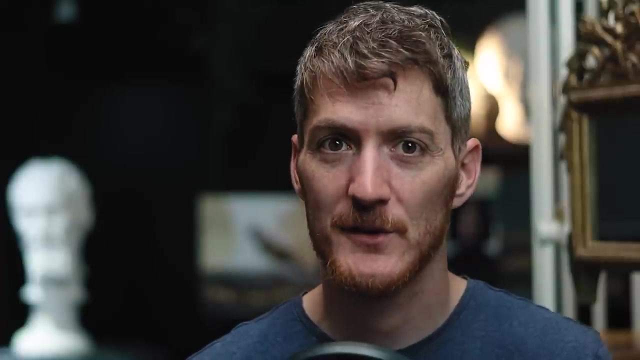 chromatic composition, and it can therefore be modified at will or even removed. It doesn't really fundamentally changes the structure of the painting. It's just there to make it more exciting and vibrant, but it's optional. By playing with these three elements, you can create all sorts of harmonies and 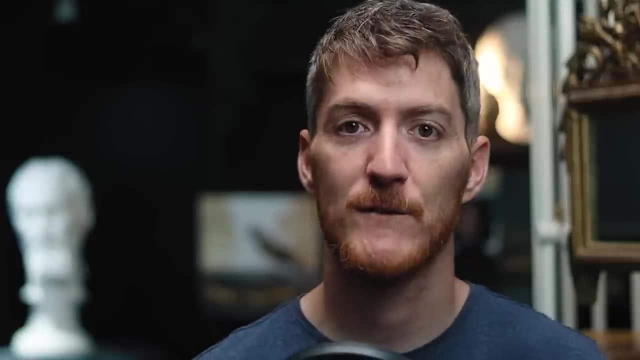 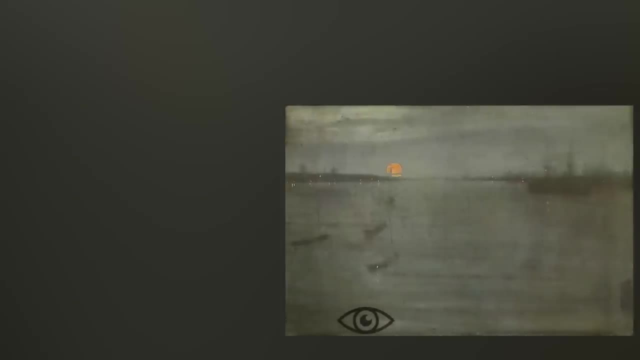 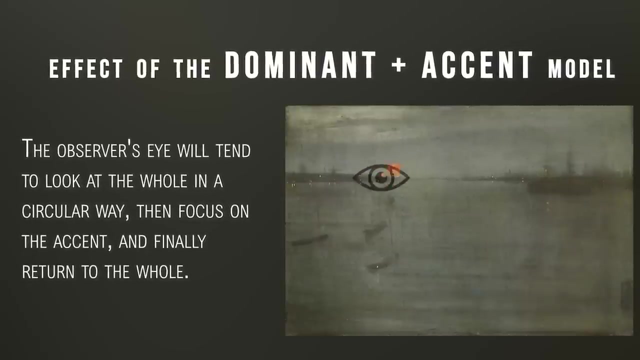 most importantly, you can need the attention of the viewers where you want it. For example, in a painting with only a dominant and an accent like this one, the observer's eye will tend to look at the hole in a circular way. then focus on. 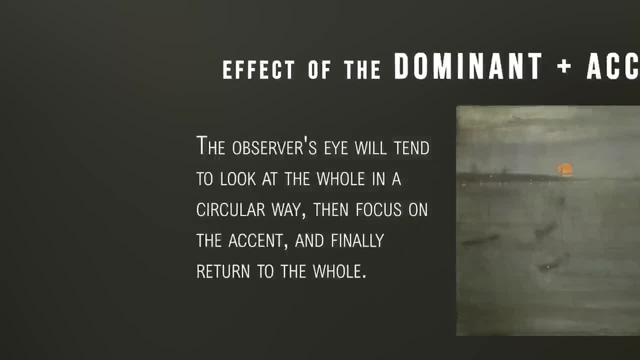 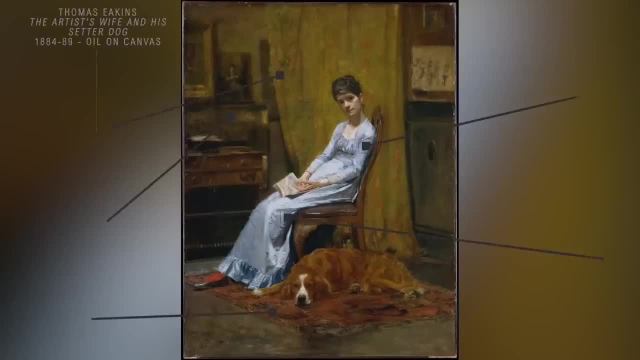 the accent, and then the accent, And finally return to the hole. Another example: when there is a dominant and a tonic, like in this painting, the tonic color is the main color. it's the one that sets the tone of the painting. the most important one, However, it's not the space. 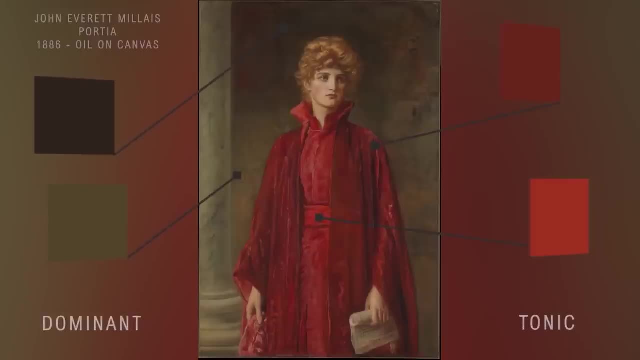 it occupies. that defines it, but its importance in the painting as a whole. To put it simply, the tonic is the color that you keep in mind when you recollect memories of the painting. The dominant completes the tonic by offering it a neutral context on which it can be fully revealed. 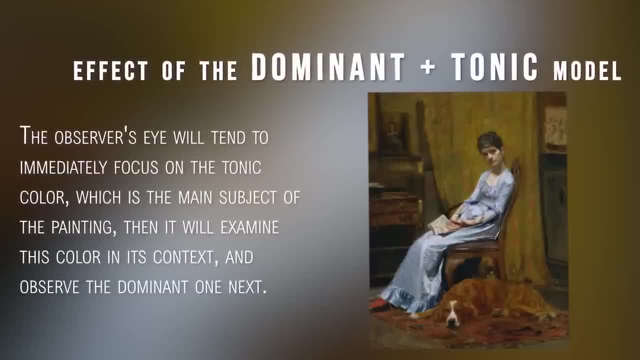 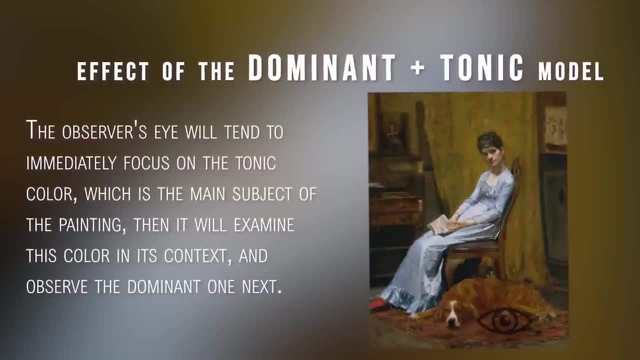 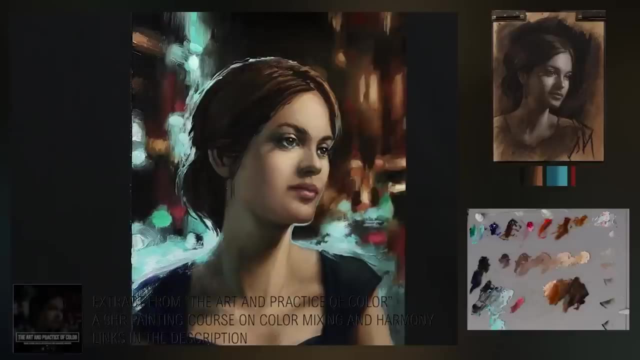 The observer's eyes will tend to immediately focus on the tonic, which is the main subject of the painting, and it will observe the dominant next. so first it will focus on the main subject and then see the picture as a whole. In this portrait painted by yours truly, yellow-brown is the dominant color. it takes the most. 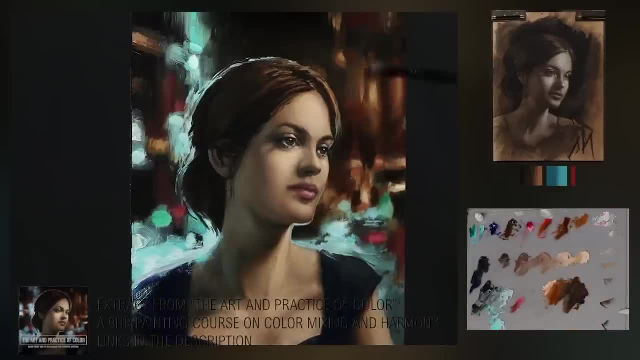 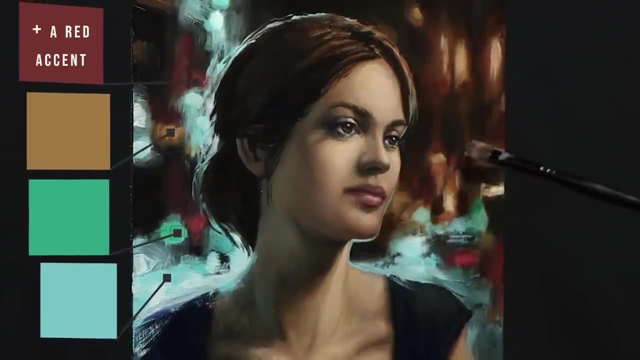 space. if you include skin tones and the strong cyan is the tonic, that's the color that's supposed to stick in your head. I have a warm light coming from the right and, in the background, a very bright blue cyan coming from the left. 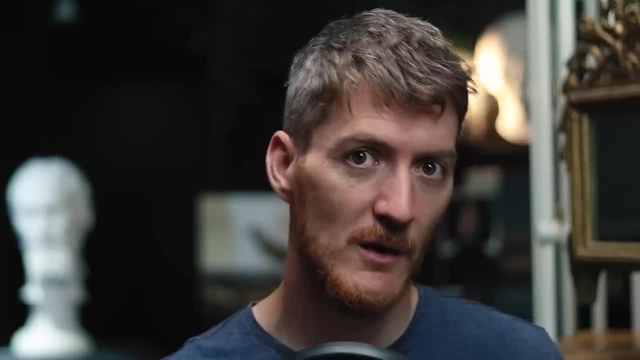 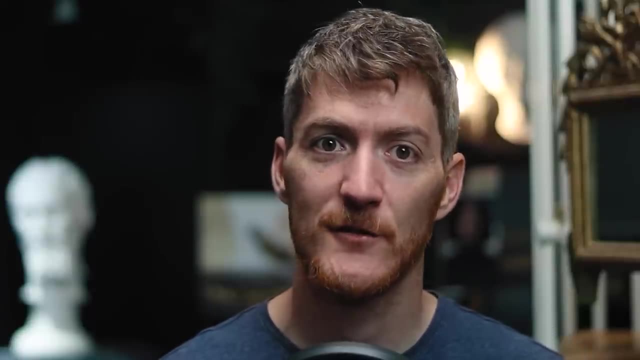 Let's now see how these notions can apply to a famous composition rule used in movies, video games and digital art actually originates from interior design. This rule does not exist in the case of paintings. In her work, she uses the idea of the whole: If you're drawn to the whole, you are drawn to the whole. 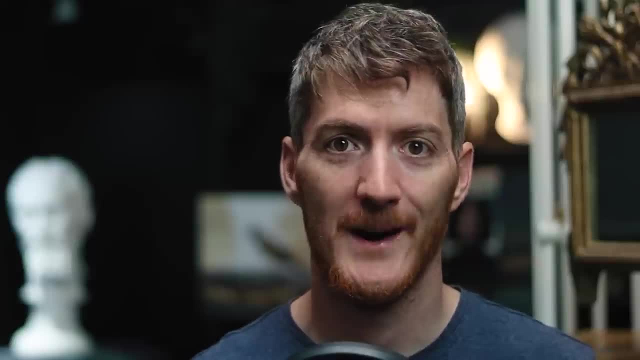 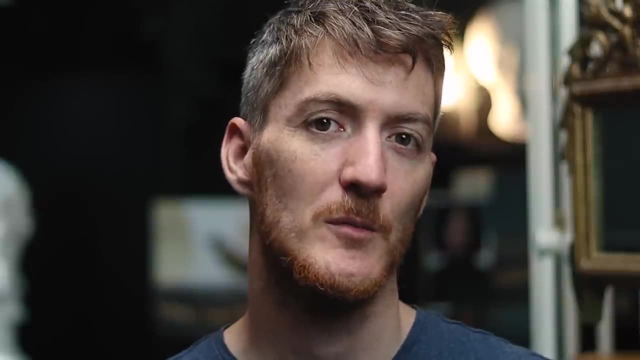 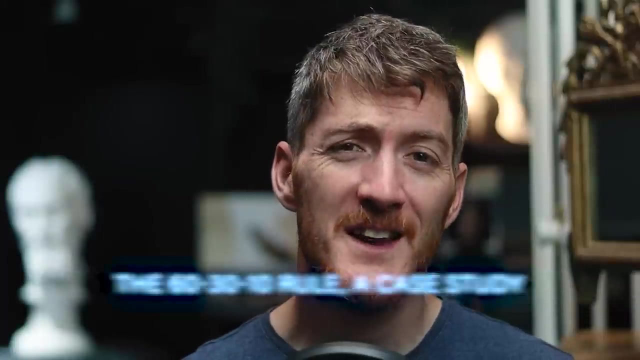 actually use the term tonic, dominant or accent. in fact, I'm the only one to use these, because I actually came up with this, but the idea is pretty similar in a way. This rule is usually known as the 60-30-10 rule. The 60-30-10 rule is not. 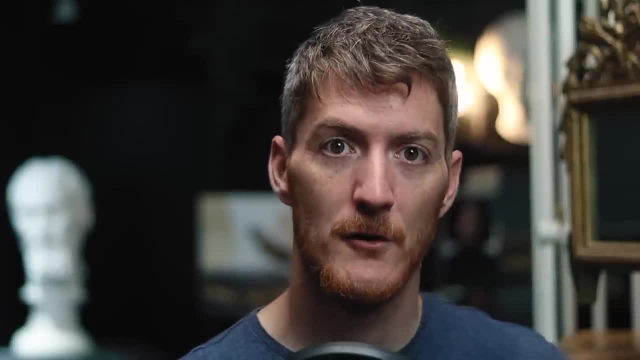 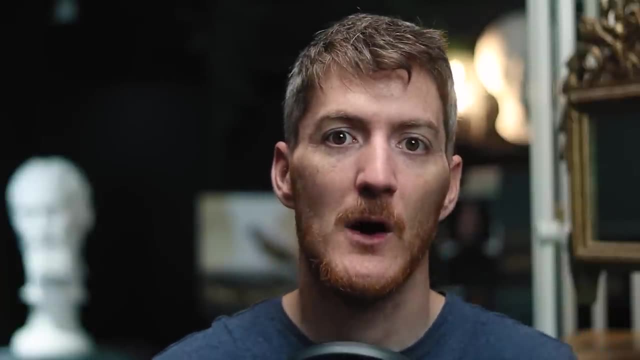 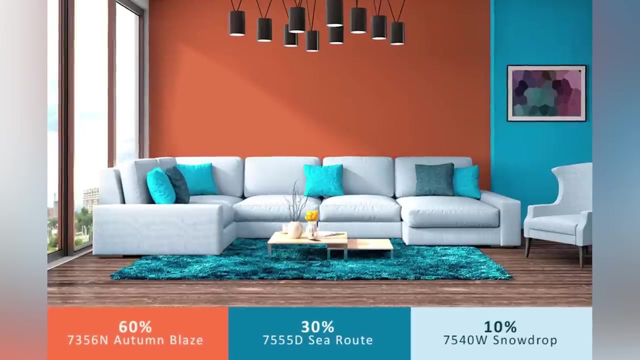 the same thing as what I call accent dominant tonic. it's only one application of what those three notions can do together, but this well-known compositional rule that I didn't invent can help and demonstrate how these notions apply. So in interior design, as well as in all the other fields, it 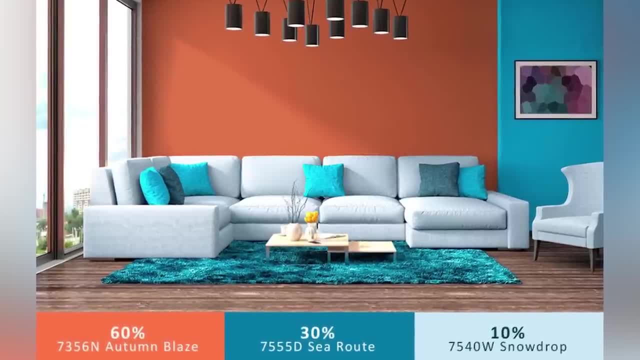 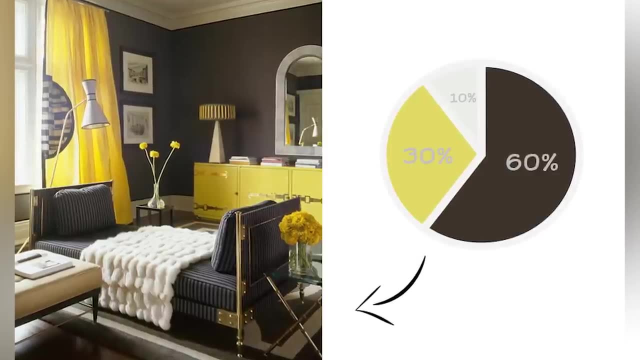 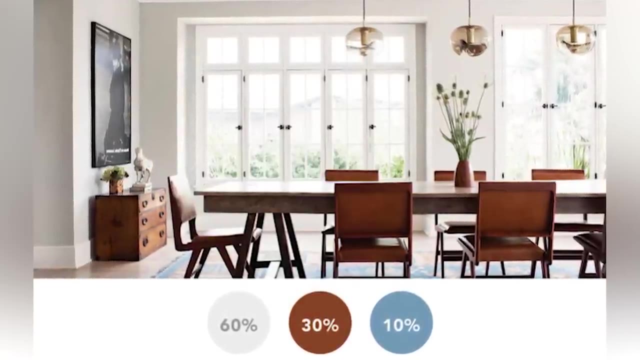 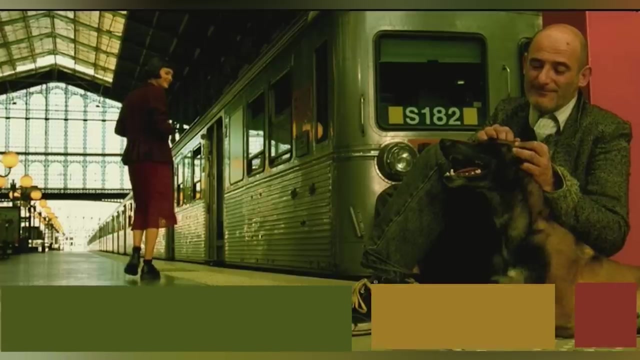 applies in. the 60-30-10 rule suggests that you should occupy 60% of a space with a rather neutral dominant color, 30% of a secondary color and 10% of an accent shade. This rule has been theorized by decorators in recent times, but it's also widely used in movies and TV shows. 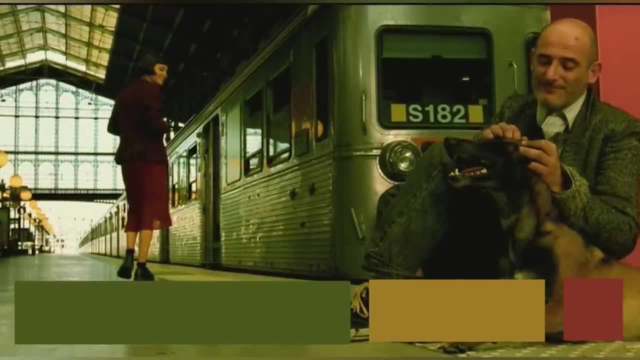 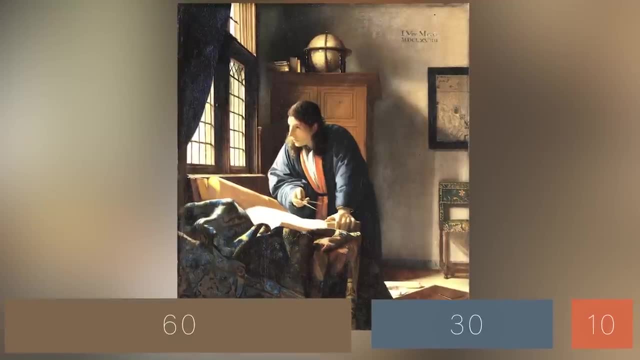 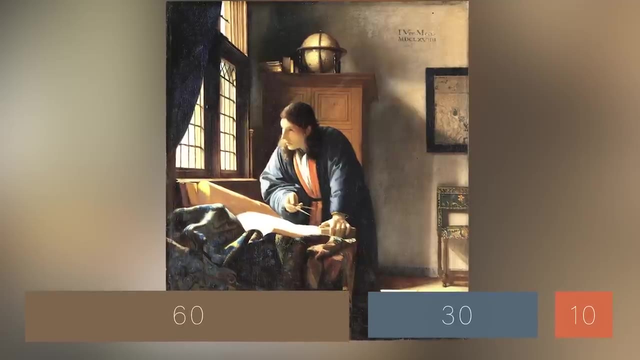 and even though it wasn't theorized as such in the history of art, you can see examples of how it applies, like with this painting by Vermeer the geographer. In this image, 60% is this beige brown background. In my color system, this is: 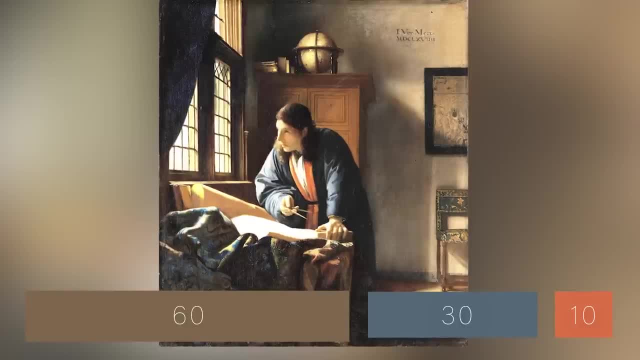 what I would call the dominant 30% is the deep blue of the coat of the geographer, also visible in the background. This is the color that I would call the dominant 30% is the deep blue of the coat of the geographer also visible. 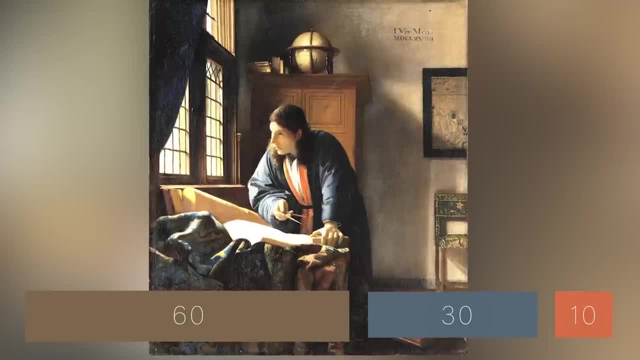 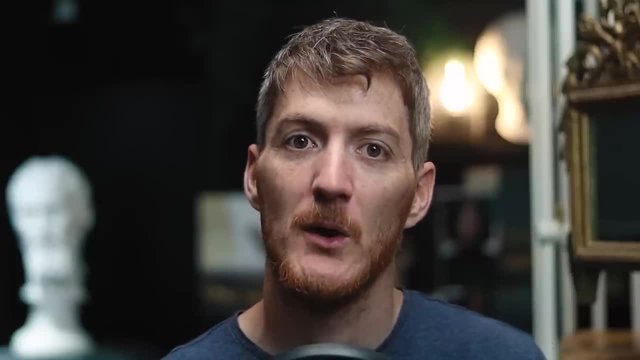 in the curtains, what I would call the tonic. and finally, the accent of the 10% is the small touch of red. here We can also see how this model creates a harmonious palette in this painting, the stone pickers by George Clausen. 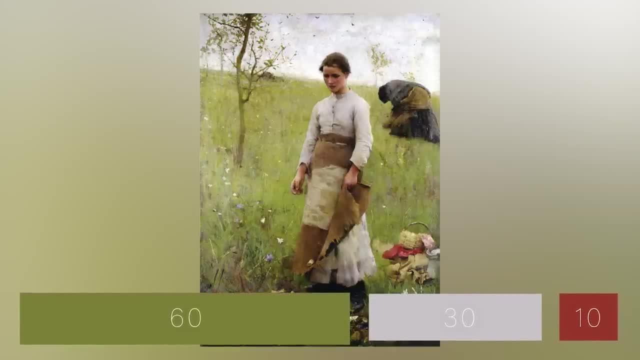 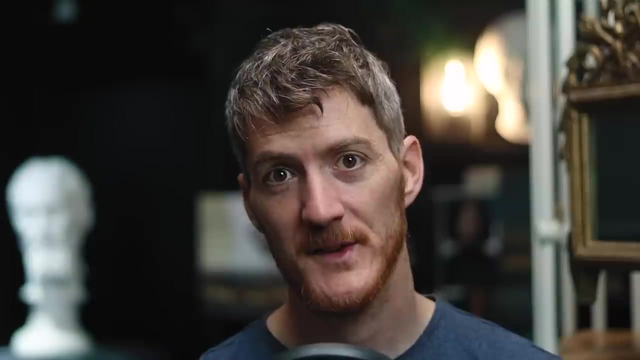 The dominant, or 60, is the light green of the fields, the tonic, or 30, is the light beige of the linen dress and the overcast sky. and finally, the accent, or 10, is the, the red piece of fabric on the right. Now, I'm not saying that Clausen or Vermeer had this rule in mind when they created those. 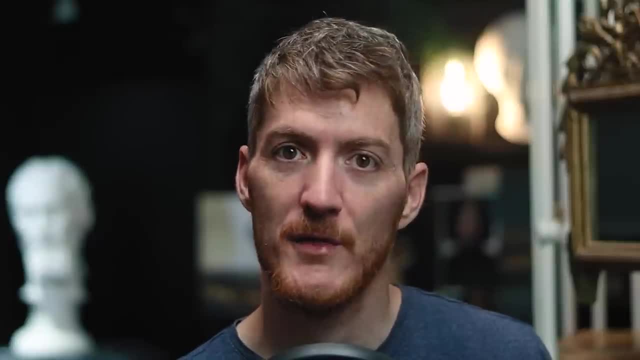 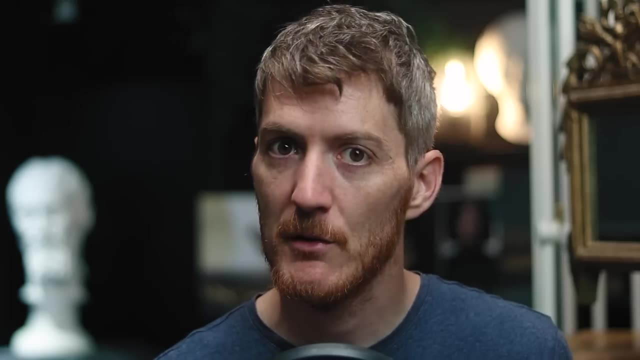 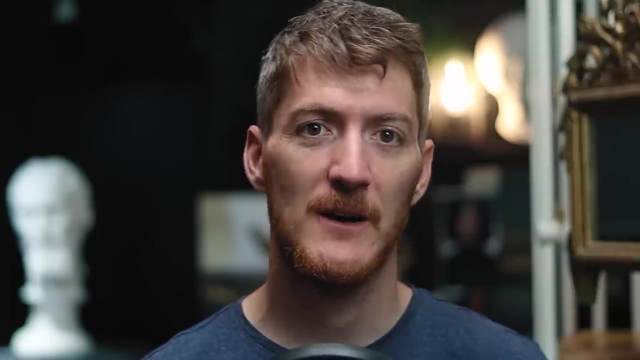 paintings. In fact, they most likely followed their intuition, but it has still led them to produce very harmonious and elegant compositions. The 60-30-10 rule is not the only rule to produce color harmony, of course. It's only one application of the notions of dominant tonic and accent, or whatever. 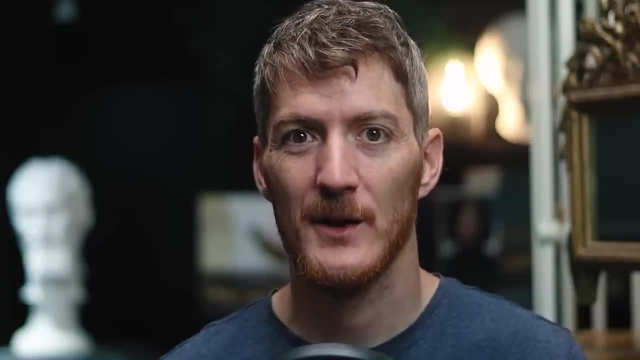 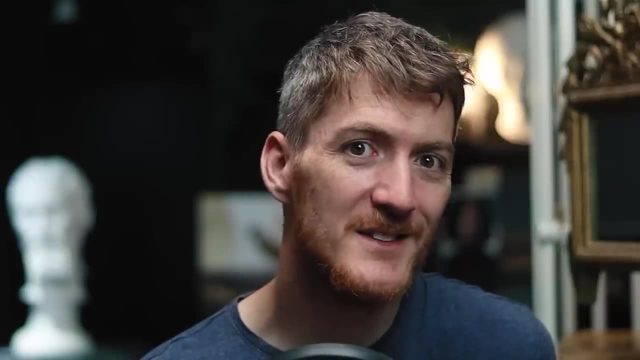 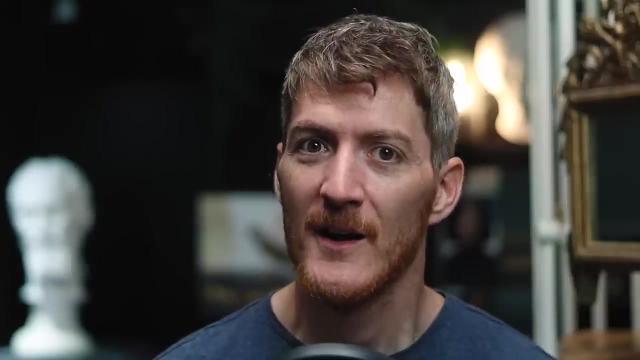 you want to call them. really, In the end they're just another way to say that colors can't all be at the same level of intensity depending on the space they occupy and their importance in the composition of the painting as a whole. Color harmony rarely comes when colors are all equally vivid next to each other, which 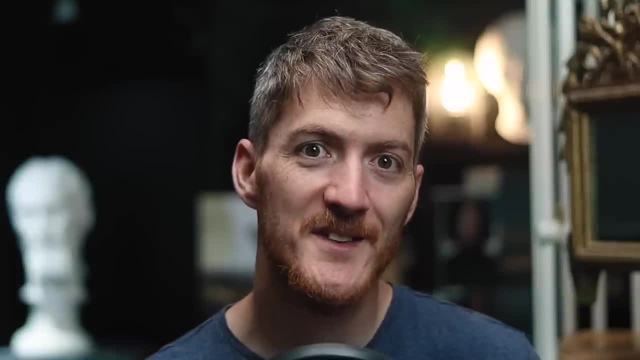 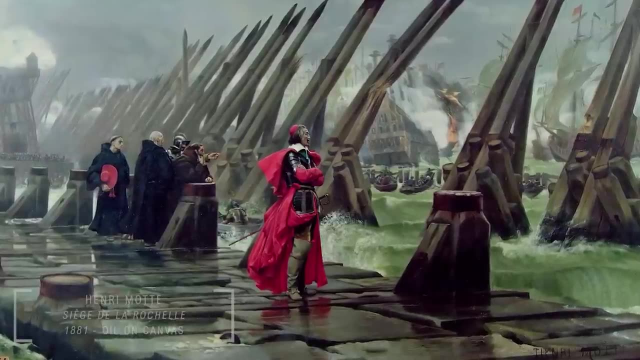 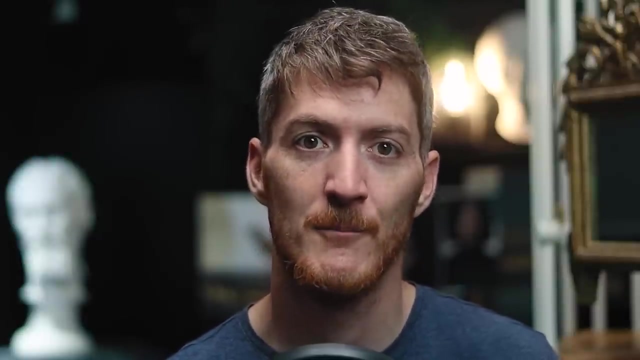 creates. color Harmony is more easily achieved if one color keeps a low profile to allow the others to capture the attention. There are many ways to explore color harmony, based on the notions of dominant tonic and accent. You can rearrange them however you like, or ignore them completely, and trust your instincts. 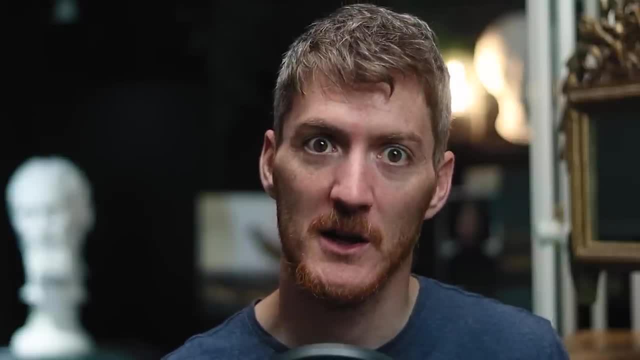 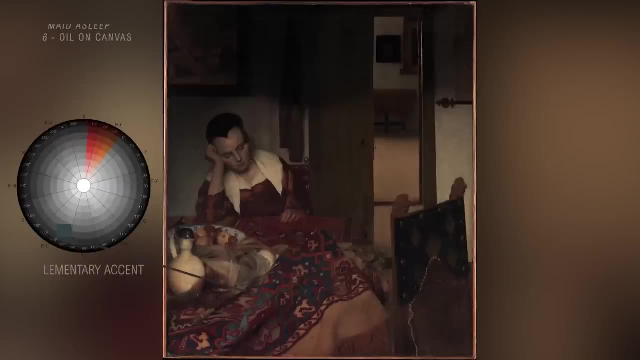 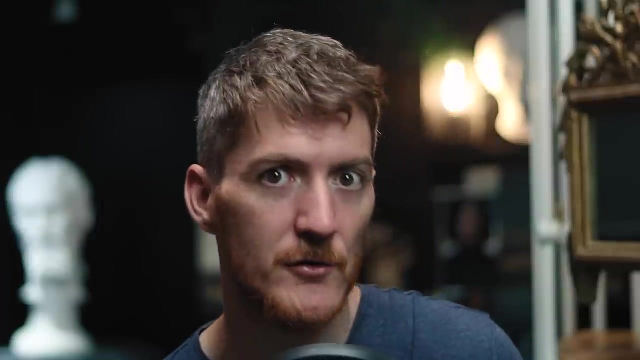 That's fine too. you can even play with disharmony. I'm sure you'll be able to use all of them. Keep in mind that it's generally better to avoid saturating the color composition too much. Neutral colors, cool and warm grays and browns allow the highlight to pop up. 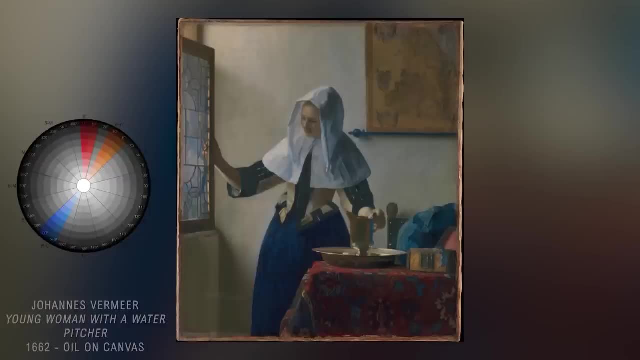 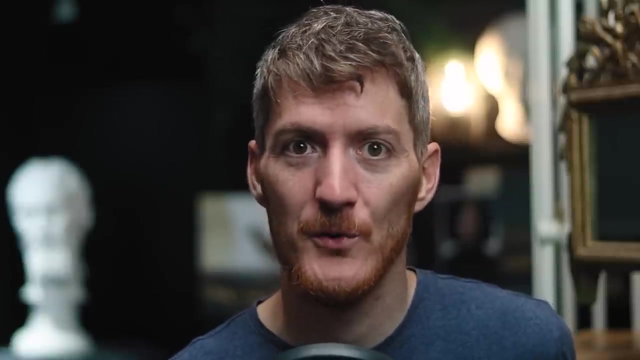 Take advantage of the almost infinite variety of low-chroma nuances and keep the most intense colors for a few well-chosen areas. That being said, nothing is stopping you from breaking the rules and creating imbalance and disharmony. The only limit, to be honest, is your imagination. 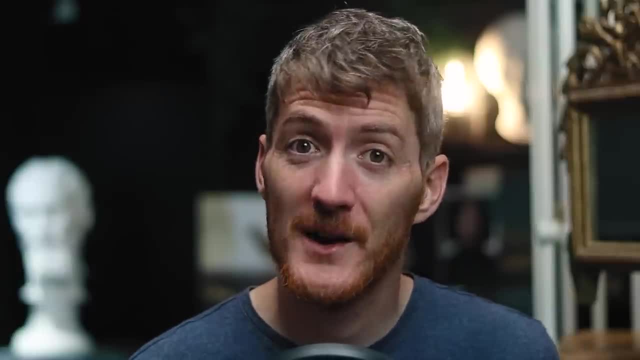 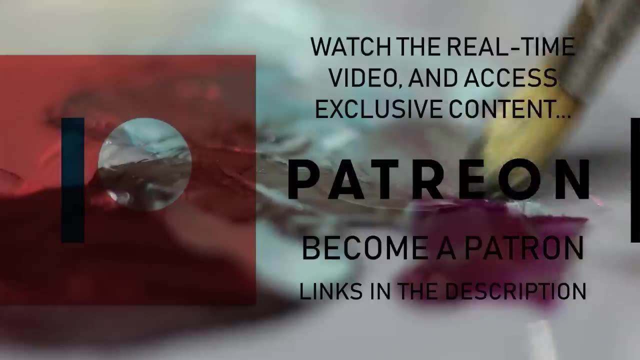 Alright, that's going to be it for this video. If you liked it, remember to leave a thumbs up and subscribe to support the channel. Again, a huge thank you to my Patreon members. This video wouldn't be possible without the amazing support. If you want to join the community, you can do so by clicking on the link in the description. If you want to support the channel, you can do so by clicking on the link in the description. If you want to support the channel, you can do so by clicking on the link in the description. 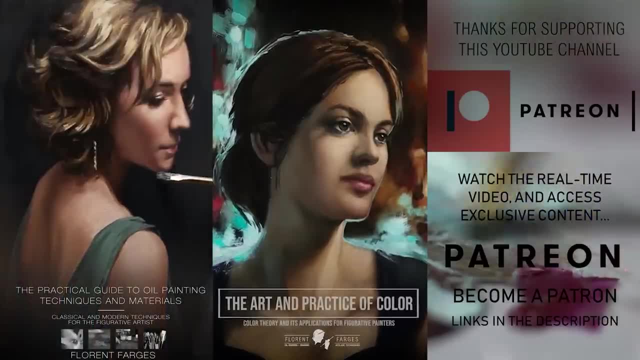 If you want to support the channel, you can do so by clicking on the link in the description. You will find the link in the description below. You will also find the link to both my courses- my Oil Painting course and my Cutter course. 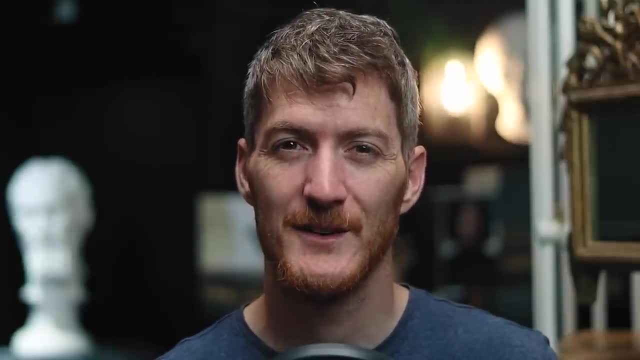 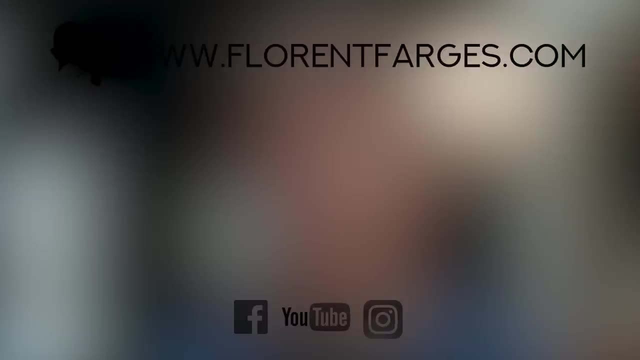 Alright, that's it for today. As always, my friends, joy and inspiration to you Bye. Thanks for watching.